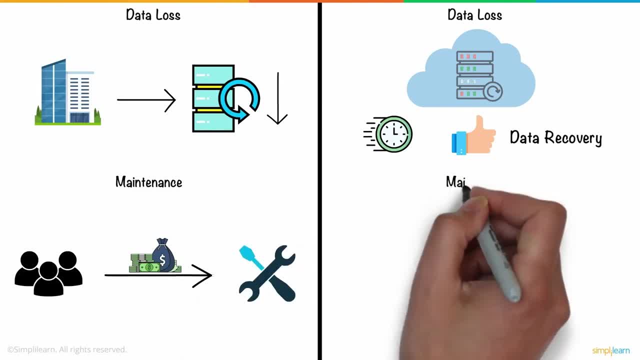 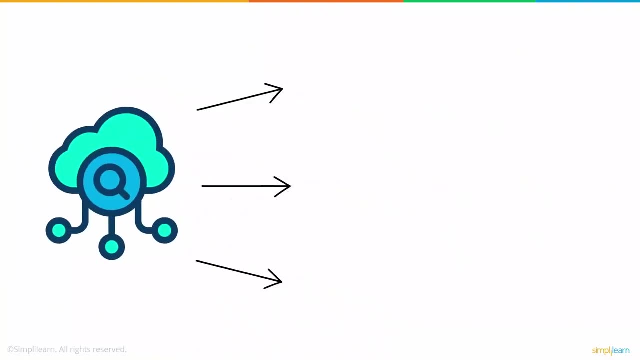 loading up the costs by a considerable degree. Cloud computing systems, on the other hand, are maintained by the cloud service providers, reducing your costs and resource allocation substantially. So now, thinking that cloud computing is a better option, you decide to take a closer look at what exactly cloud computing is. Cloud computing refers to the 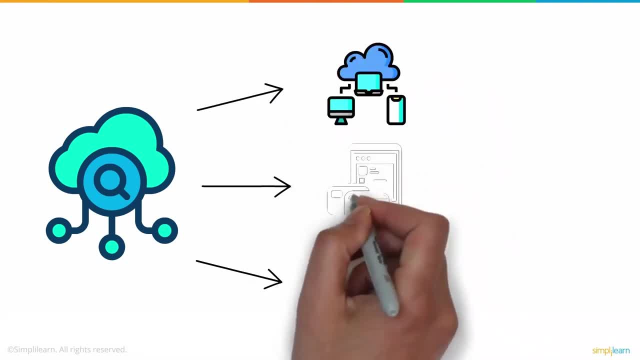 delivery of on-demand computing services over the internet on a pay-as-you-go basis. In simpler words, rather than managing files and services on a local storage device, you'll be doing the same over the internet in a cost-efficient manner. Cloud computing has two types of models – deployment. 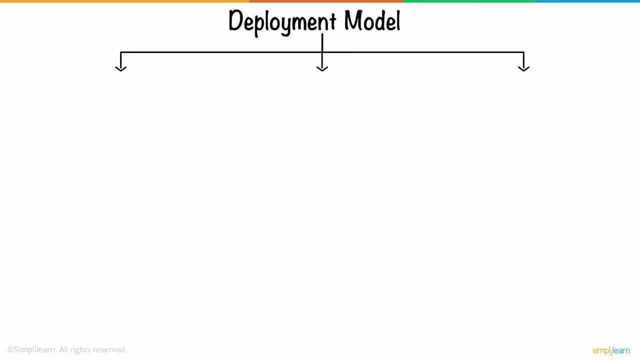 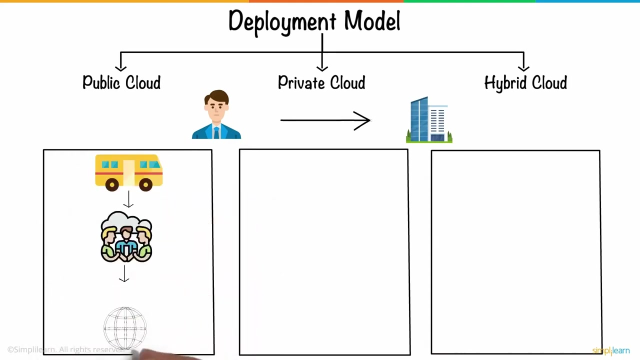 model and service model. There are three types of deployment models – public, private and hybrid cloud. Imagine you're traveling to work. You've got three options to choose from. One you have buses, which represent public clouds. In this case, the cloud infrastructure is available. 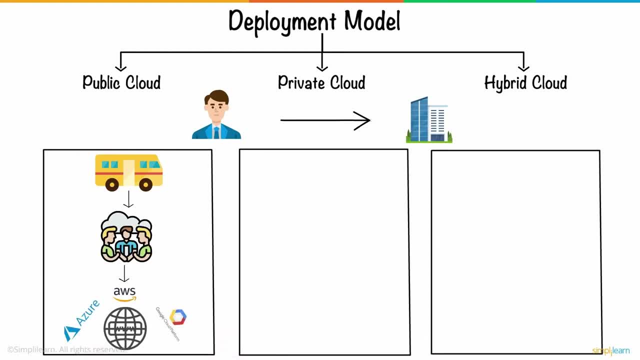 to the public over the internet. These are owned by cloud service providers. Two, then you have the option of using your own car. This represents the private cloud. With the private cloud, the cloud infrastructure is exclusively operated by a single organization. This can be managed by the. 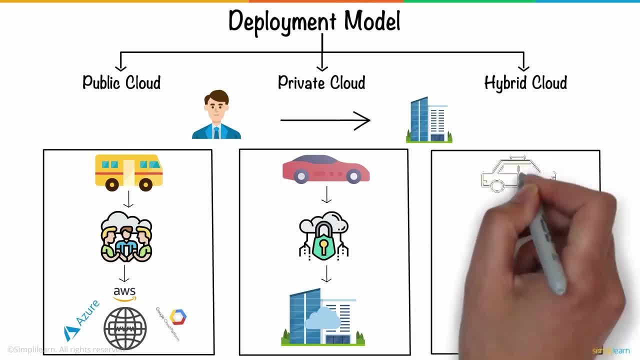 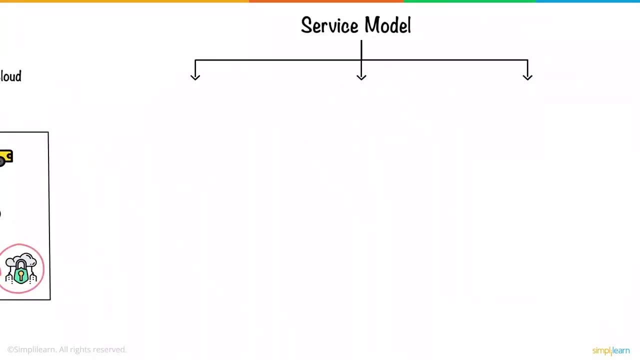 organization or a third party. And finally, you have the option to hail a cab. This represents the hybrid cloud. A hybrid cloud is a combination of the functionalities of both public and private clouds. Next, let's have a look at the service models. There are three major service models. 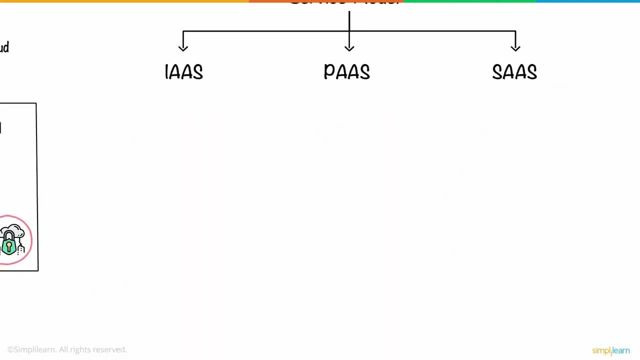 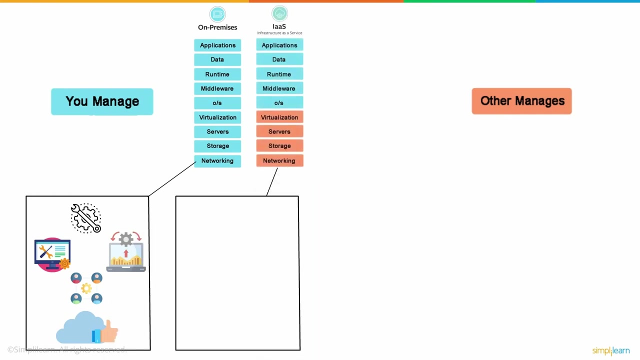 available – EAS, PaaS and SaaS. Compared to on-premise models, where you'll need to manage and maintain every component, including applications, data virtualization and middleware, cloud computing service models are hassle-free. IaaS refers to infrastructure as a service. It. 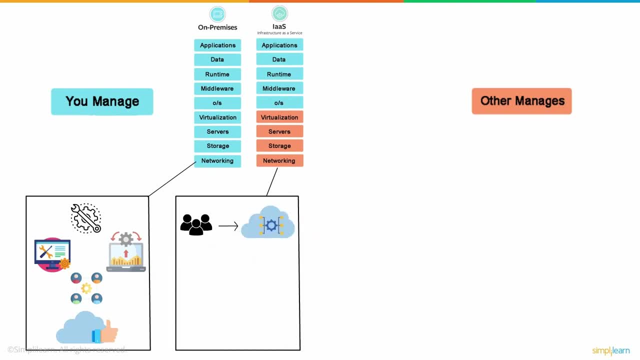 is a cloud service model where users get access to basic computing infrastructure. They are commonly used by IT and cloud services. They are also used by IT and cloud services. They are commonly used by IT and cloud services. They are also used by IT and cloud services. They are also used by IT and. 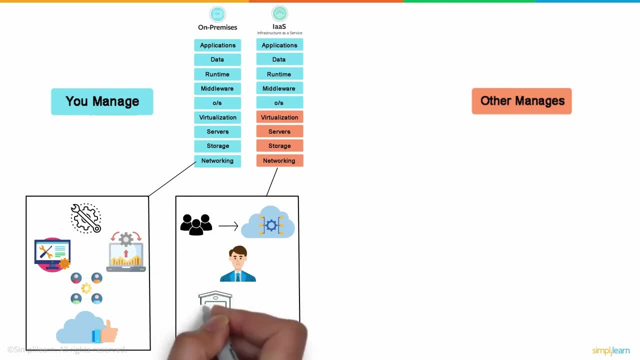 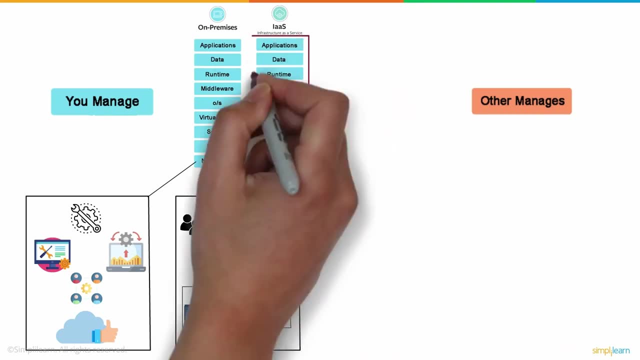 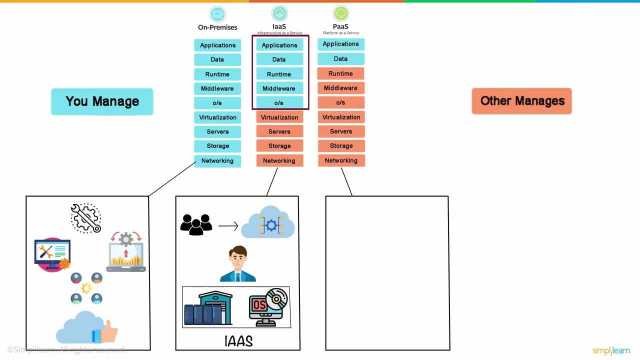 IT administrators. If your organization requires resources like storage or virtual machines, IaaS is the model for you. You'll only have to manage the data runtime, middleware applications and the OS, while the rest is handled by the cloud providers. Next we have PaaS. PaaS or Platform. 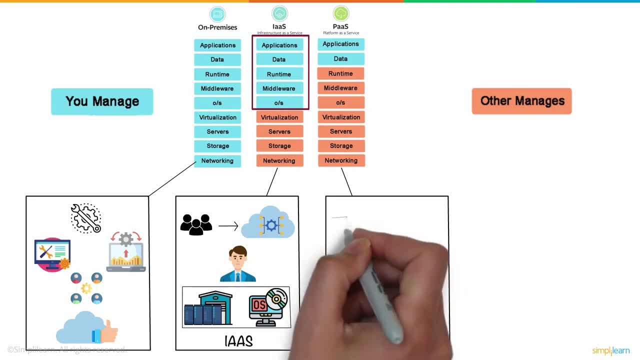 as a Service provides cloud platforms and runtime environments for developing, testing and managing applications. This service model enables users to deploy applications without the need to acquire, manage and maintain the related architecture. If your organization is in need of a platform for creating software applications, PaaS is the model for you. PaaS only requires you to 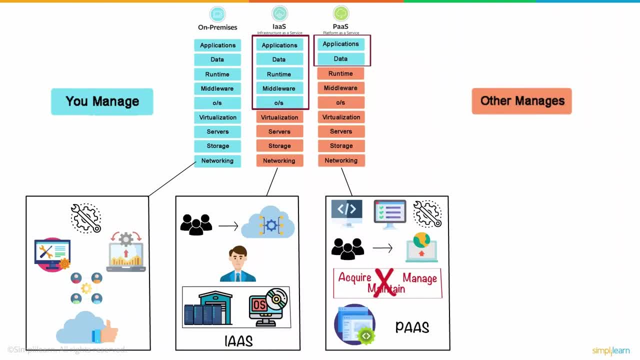 handle the applications and the data. The rest of the components, like runtime, middleware, operating systems, servers, storage and others, are handled by the cloud service providers. And finally, we have SaaS. SaaS, or Software as a Service, involves cloud services for hosting and managing your 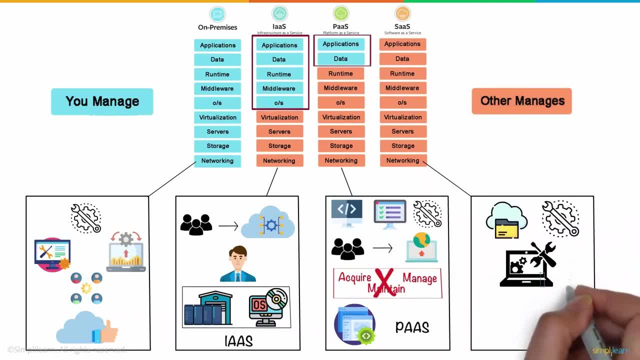 software applications. PaaS is the model for you. You'll only have to manage the data runtime and operations. Software and hardware requirements are satisfied by the vendors, so you don't have to manage any of those aspects of the solution. If you'd rather not worry about the hassles of owning, 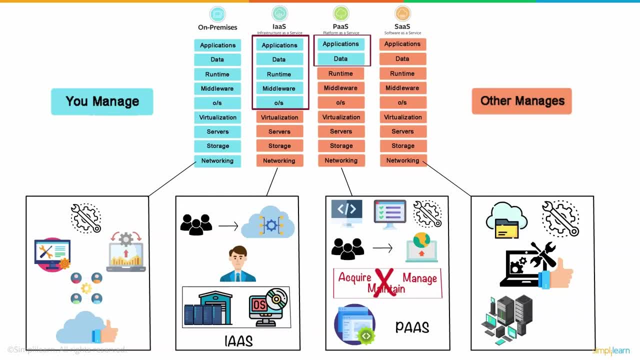 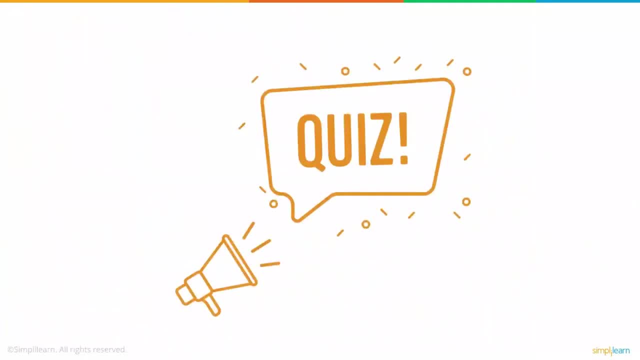 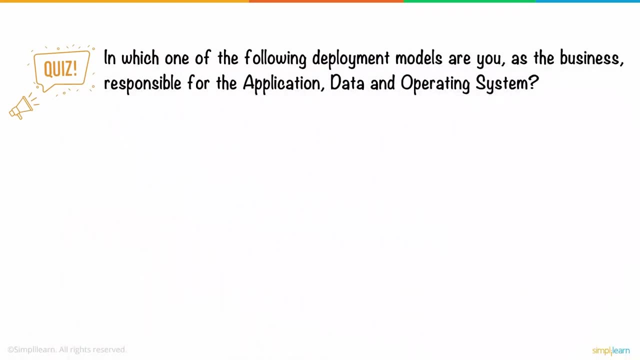 any IT equipment, the SaaS model would be the one to go with. With SaaS, the cloud service provider handles all components of the solution required by the organization. Time for a quiz now. In which of the following deployment models are you, as the business, responsible for the application data? 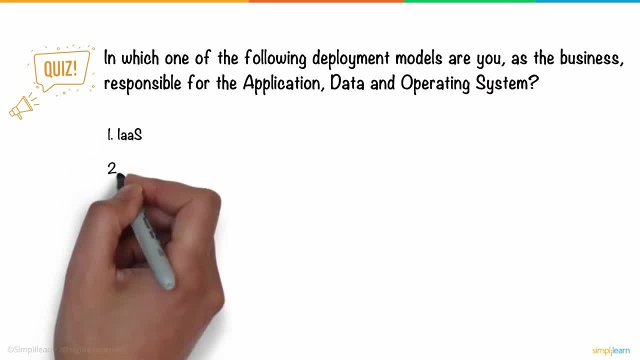 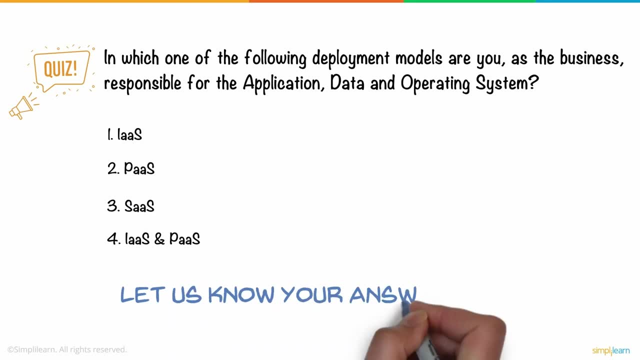 and operating system. If you're a business, you're responsible for the application, data and operating system: One IaaS, Two PaaS, Three SaaS, Four IaaS and PaaS. Let us know your answer in the comment section below. 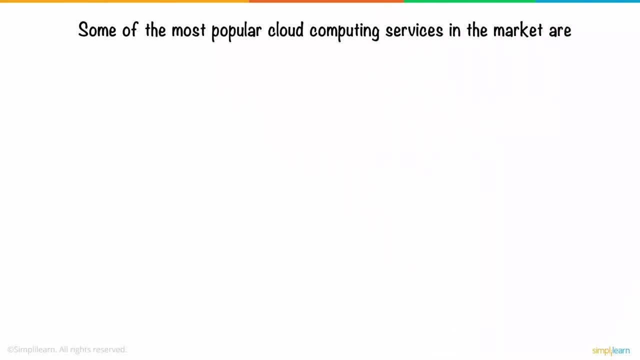 Coming back to cloud computing, some of the most popular cloud computing services in the market are AWS or Amazon Web Services, Microsoft Azure and Google Cloud Platform. Want to learn more about them and how they differ from each other. Click on the top right corner for an analysis of how. 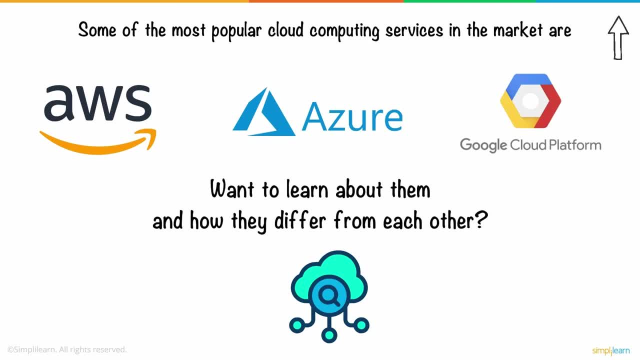 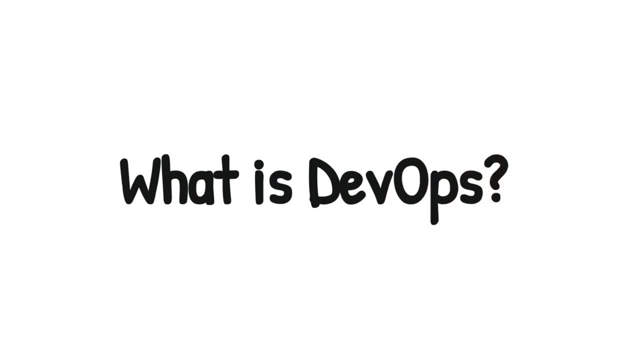 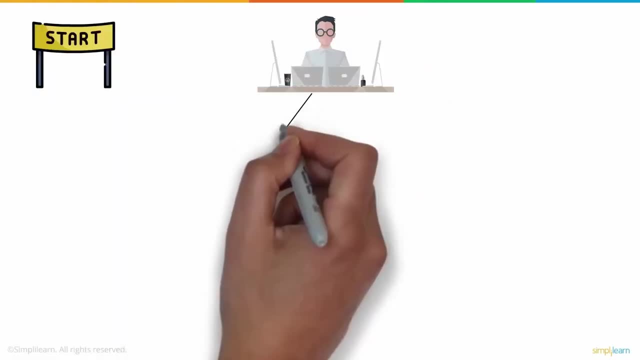 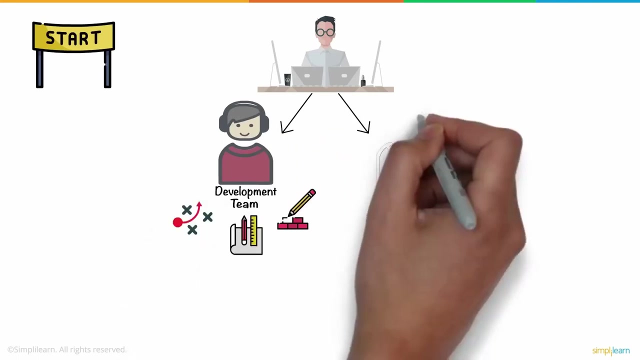 they differ from each other. We hope you found this informative and helpful. Right from the start, software development comprised two different departments: The development team that develops the plan, designs and builds the system from scratch, and the operation team for testing and implementation of whatever is developed. The 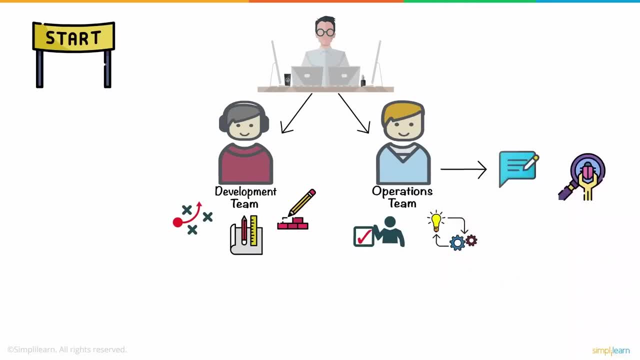 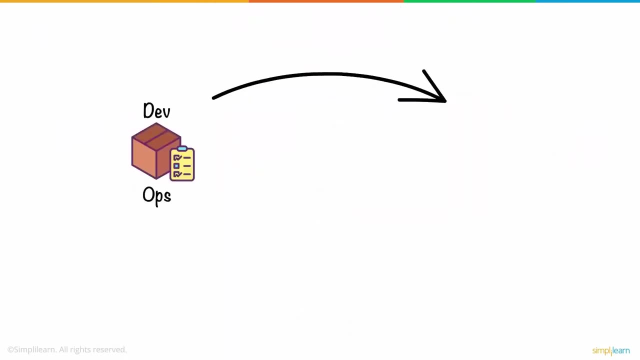 gave the development team feedback on any bugs that needed fixing and any rework required. Invariably the development team would be idle, awaiting feedback from the operations team. This undoubtedly extended timelines and delayed the entire software development cycle. There would be instances where the development team moves on to the next project. 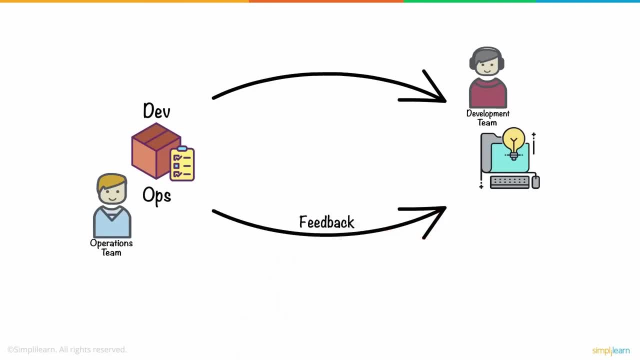 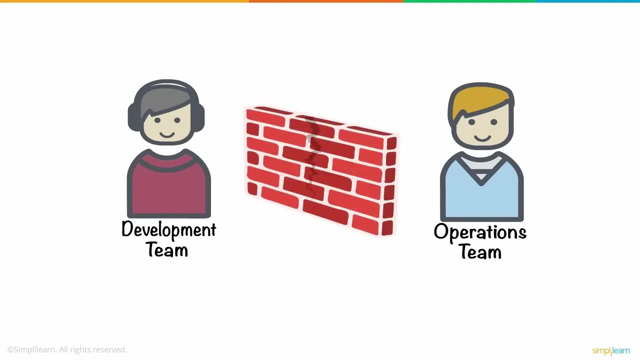 while the operations team continues to provide feedback for the previous code. This meant weeks, or even months for the project to be closed and final code to be developed. Now, what if the two departments came together and worked in collaboration with each other? What if the wall of confusion was broken? 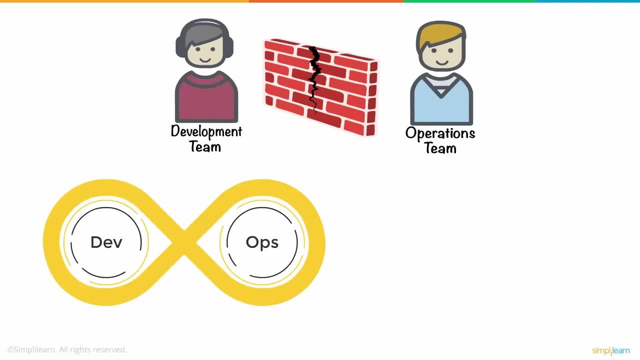 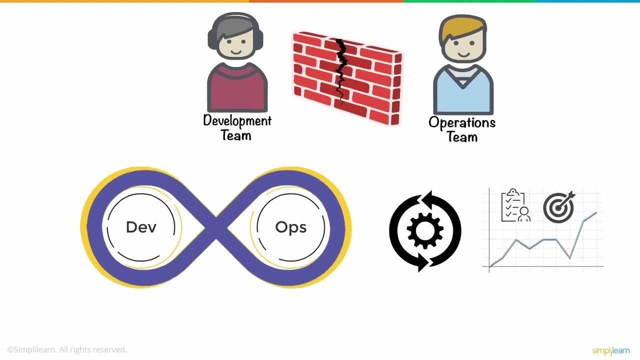 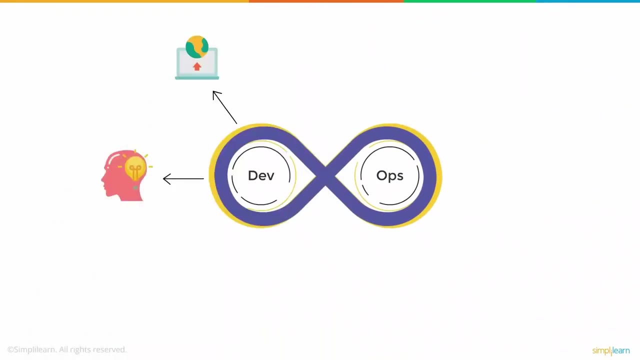 And this is called the DevOps approach. The DevOps symbol resembles an infinity sign, suggesting that it is a continuous process of improving efficiency and constant activity. The DevOps approach makes companies adapt faster to updates and development changes. The teams can now deliver quickly and the deployments are more consistent and smooth. 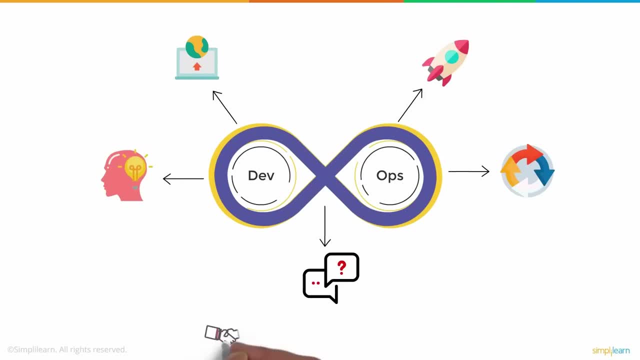 The DevOps approach makes companies adapt faster to updates and development changes. The teams can now deliver quickly and the deployments are more consistent and smooth. Though there may be communication challenges, DevOps manages a streamlined flow between the teams and makes the software development process successful. 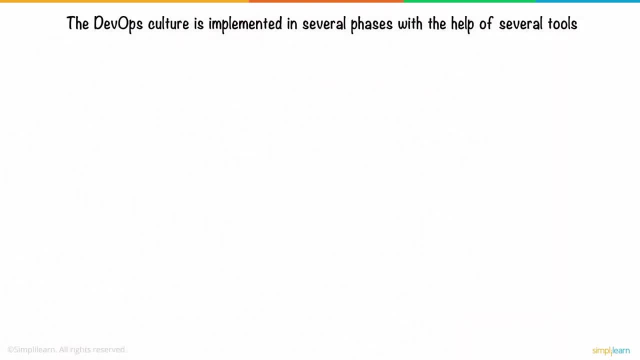 The DevOps culture is implemented in several phases with the help of several tools. Let's have a look at these phases. The first phase is the planning phase, where the development team puts down a plan keeping in mind the application objectives that are to be delivered to the customer. 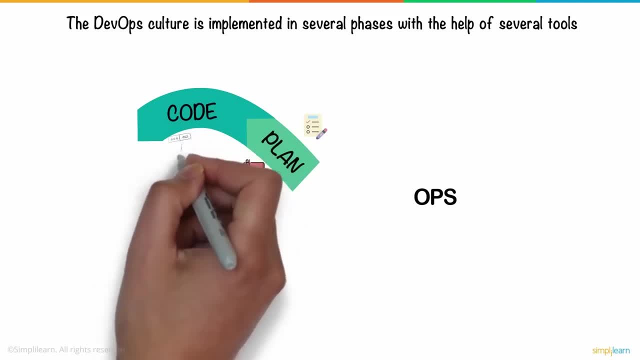 Once the plan is made, the coding begins. The development team works on the same code and different versions of the code are stored into a repository With the help of tools like Git and Merged When Required. this process is called version control. The code is then made executable with tools like Maven and Gradle in the build stage. 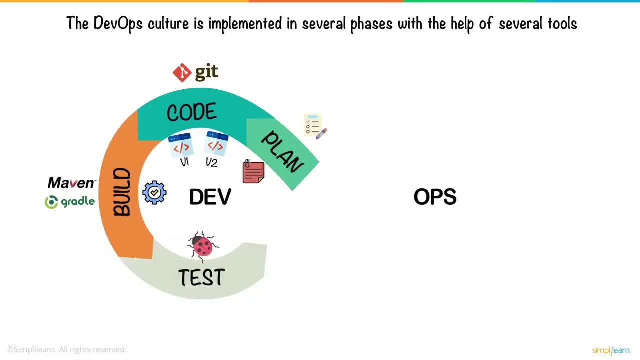 After the code is successfully built, it is then tested for any bugs or errors. The most popular tool for automation testing is Selenium. Once the code has passed several manual and automated tests, we can say that it is ready for deployment and is sent to the operations team. 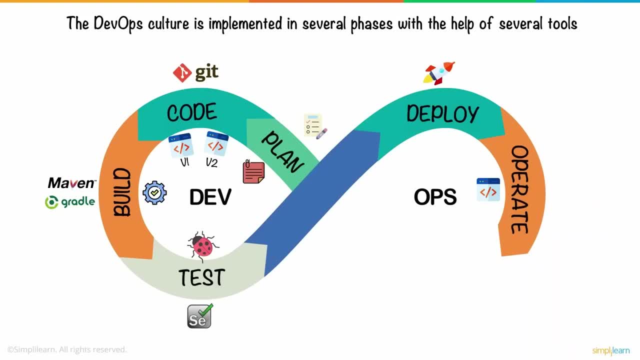 The operations team now deploys the code to the working environment. The most prominent tools used to automate these phases are Ansible, Docker and Kubernetes. After the deployment, the product is continuously monitored, and Nagios is one of the top tools used to automate this phase. 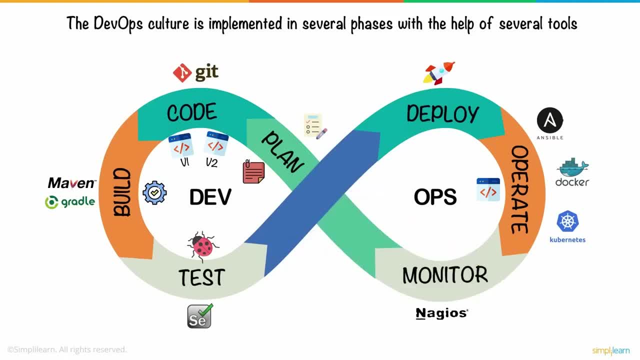 The feedback received after this phase is sent back to the planning phase, and this is what forms the core of the DevOps lifecycle, that is, the integration phase. Jenkins is the tool that sends the code for building and testing, If the code passes the test. 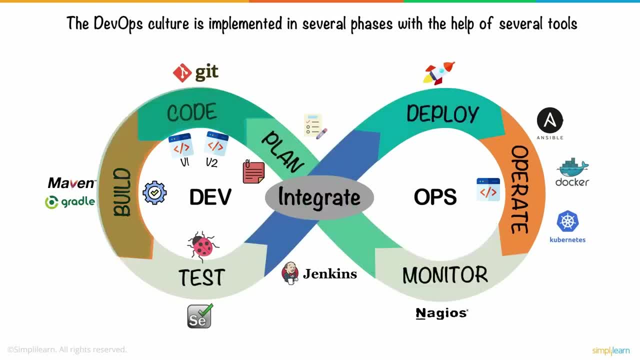 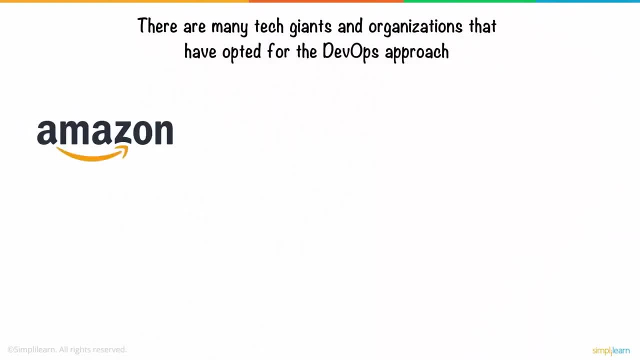 it is sent for deployment, and this is referred to as continuous integration. There are many tech giants and organizations that have opted for the DevOps approach, For example, Amazon, Netflix, Walmart, Facebook and Adobe. Netflix introduced its online streaming service in 2007.. 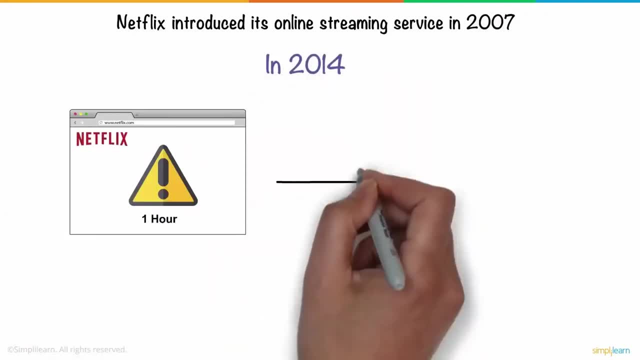 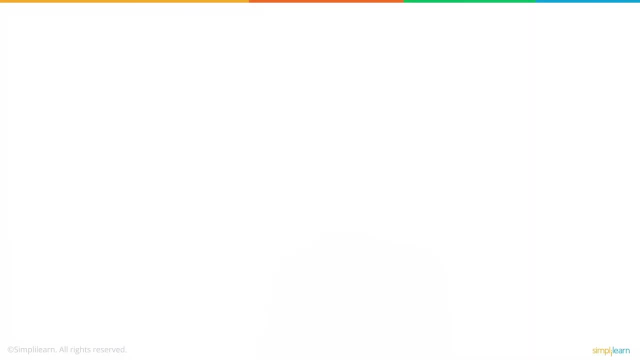 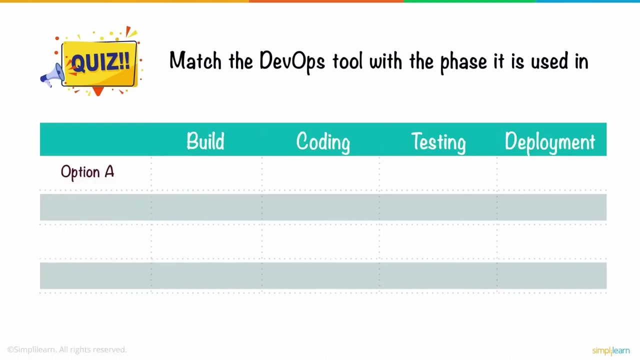 that does not fall apart when any such thing happens. So, on this note, here is a quiz for you: Match the DevOps tool with the phase it is used in: A, B, C, D. None of the above. Today, more and more companies lean towards automation, with the aim of reducing its. 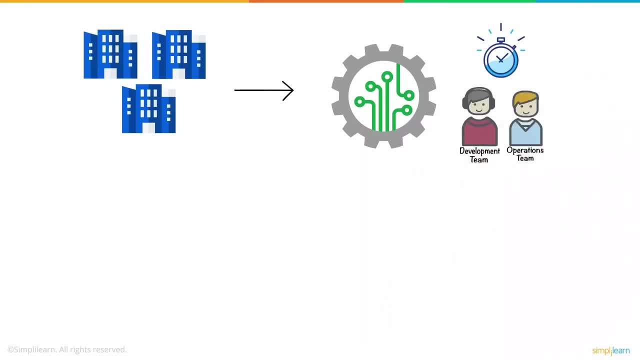 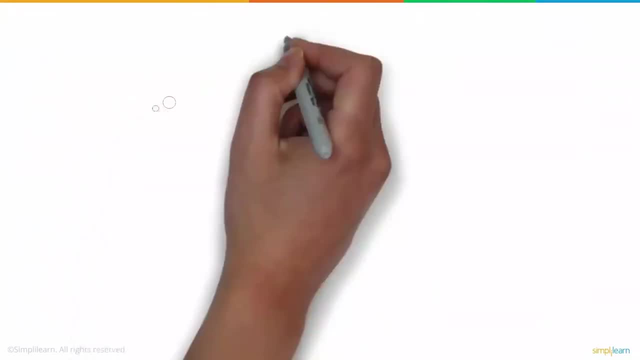 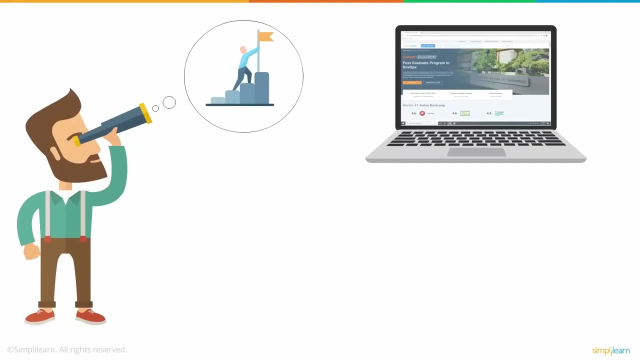 delivery time and the gap between its development and operations teams. To attain all of these, there is just one gateway – DevOps. And if you are also looking forward to doing the same and excel in DevOps, check out some of our assembly-learn's postgraduate program in DevOps Design in Collaboration with Caltech CTME. 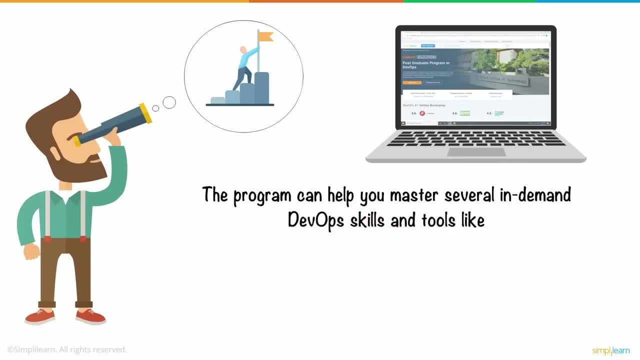 The program can help you master several in-demand DevOps skills and tools, like continuous integration and delivery, DevOps on cloud, Kubernetes, Docker and much more. We hope you enjoyed this video. If you did, a thumbs up would be really appreciated. 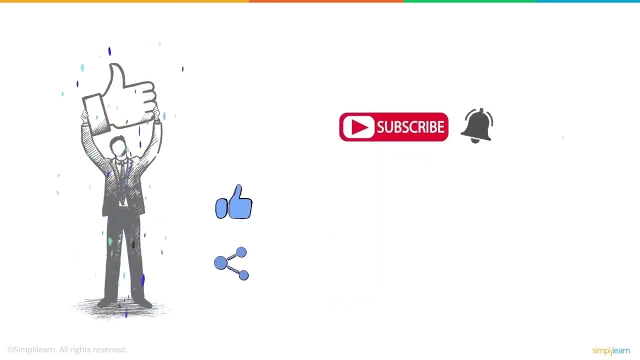 Here's your reminder to subscribe to our channel and to click on the bell icon for more on the latest technologies and trends. Thank you for watching and stay tuned for more. More from Simply Learn.